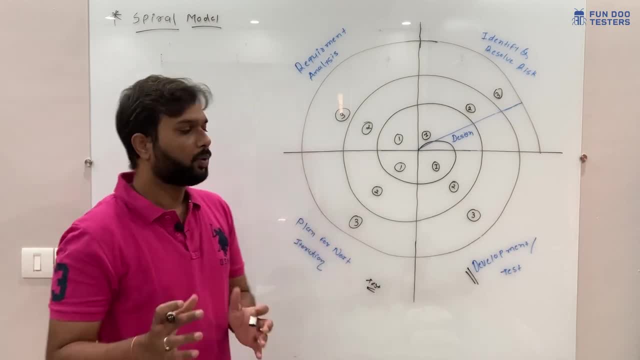 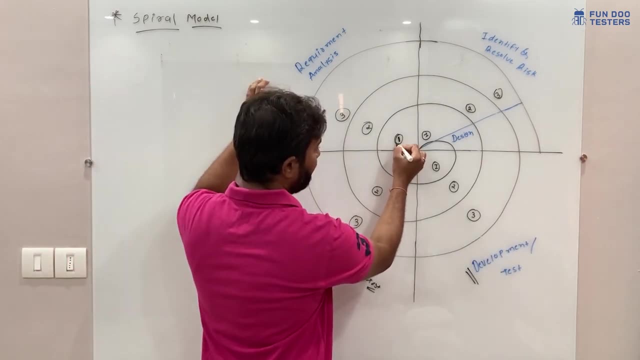 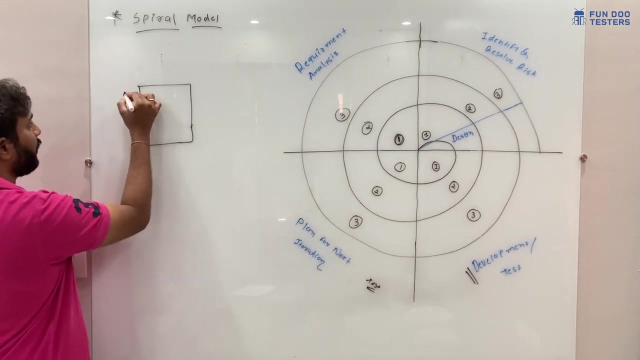 initially, whenever client will come up with the requirement. so first, in first phase, they will understand the requirement. so here first, first, this is my first iteration. in first iteration the requirement and development analysis works, so how it happens. so this is my complete product, which is 100 percent. 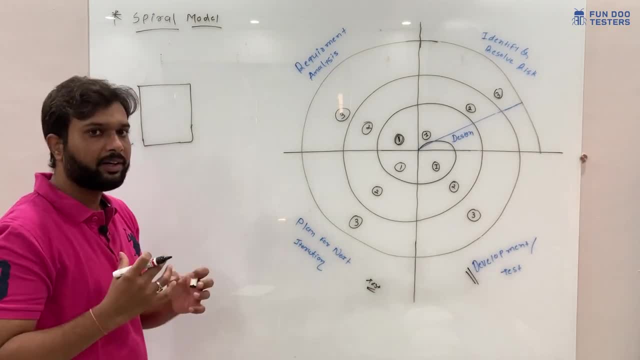 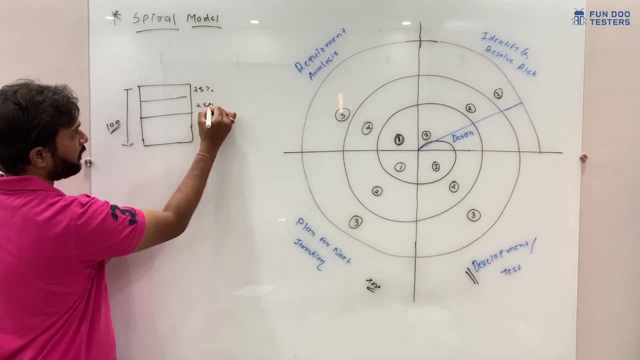 here this is 100 percent. so what they will do? they will divide into a small chunk. so here first i will check- i will take 25 percent of one chunk, then 25 percentage of second chunk. here i will take 50 percentage of third chunk. so how? 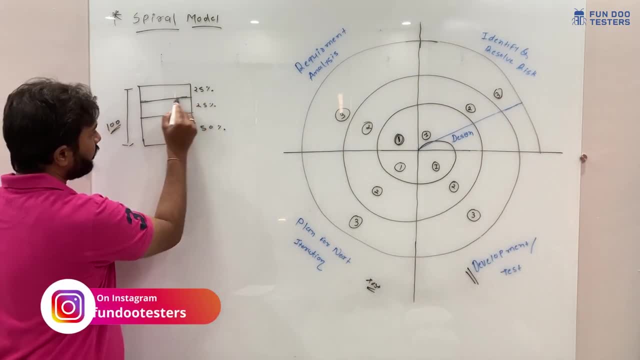 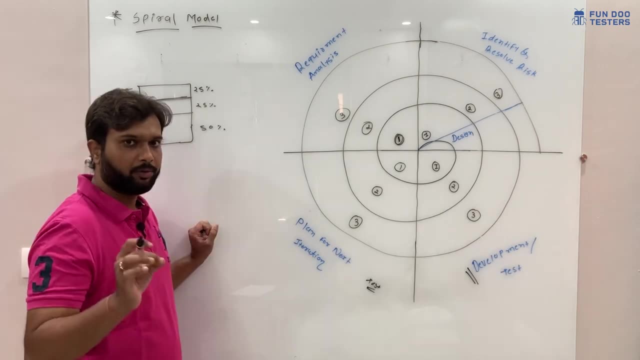 this is how it will work. so what they will do. first, they will understand only 25 percent of the product and they will do the requirement analysis of the 25 percentage of the product. if you take an example of the whatsapp, uh story feature was not there. so let's consider: 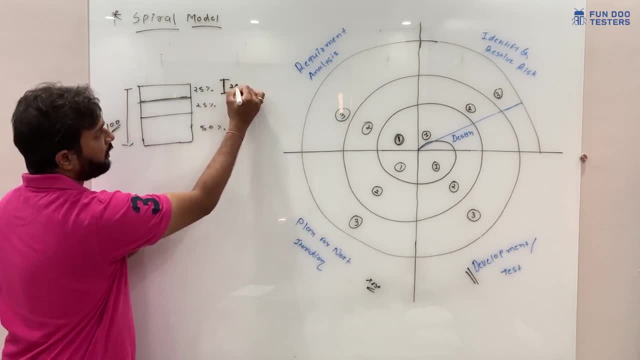 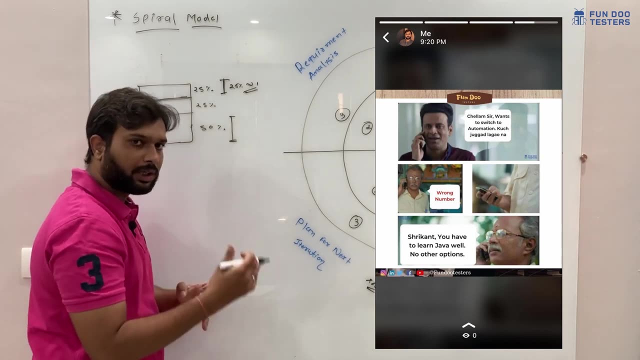 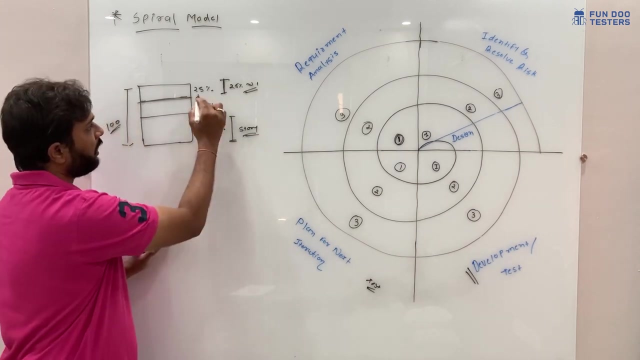 they consider they took this 25 percentage phase of whatsapp because story feature is not there. in third chunk they have developed the story feature. so this is how they have split the functionality: here they will take the story feature. so this is the real-time example now. what they will do in first 25 percentage of part they will 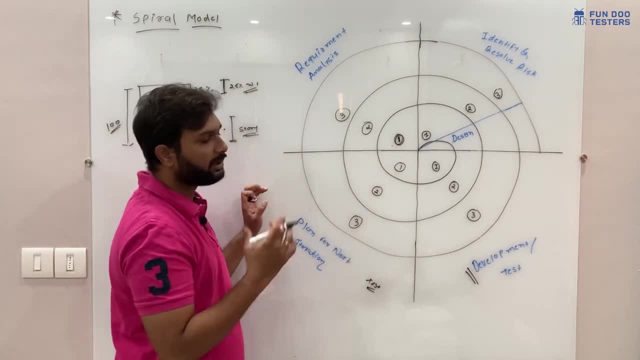 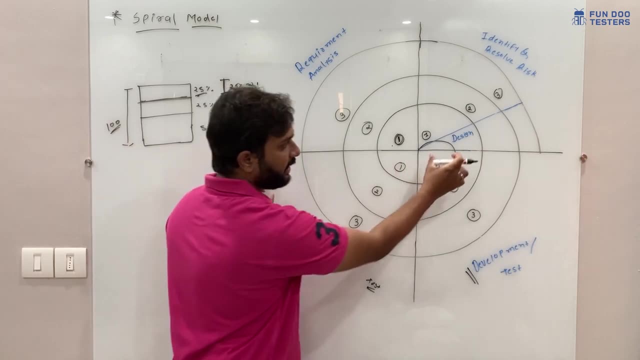 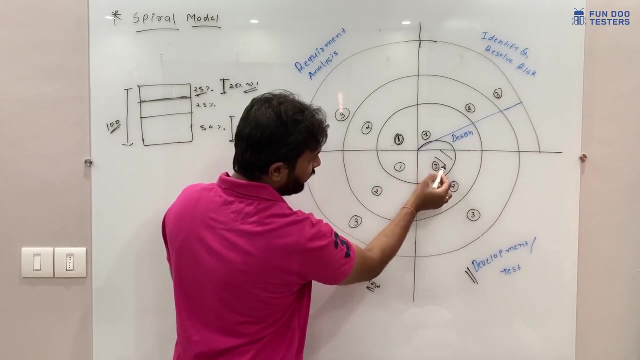 do the requirement analysis. and once requirement analysis done, they will identify the risk. and here itself they haven't given the small phase of the design, so here design phase will take place and then, once design phase is done- so in only first part, this is the only first part- they will do the development. 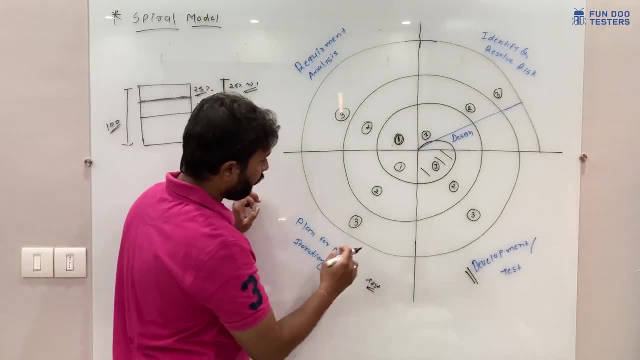 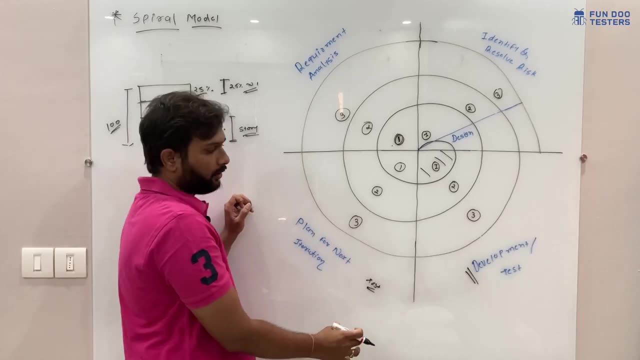 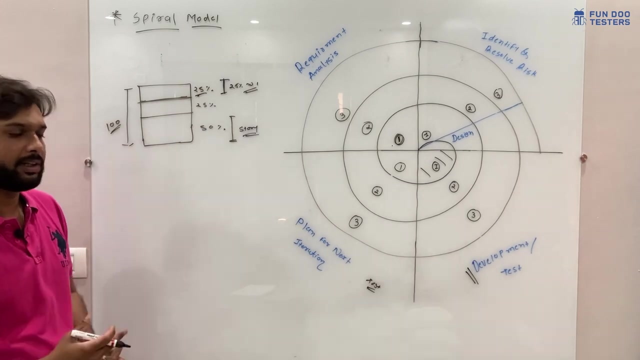 and test. once development and testing is done, it will go for the next iteration. here you can consider as a plan for the next iteration or test. if testing is pending here, testing will take place. otherwise they have to plan for the next iteration. so what they will decide. 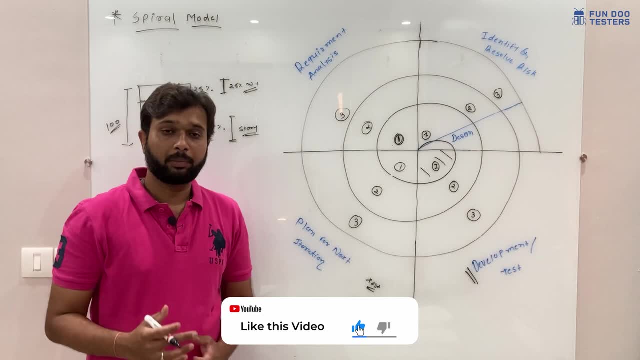 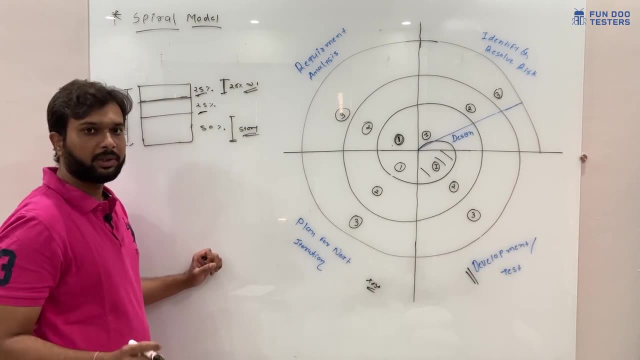 in next iteration what they are going to build or what is the plan for the next build. so in next iteration they are going to take another 25 of the chunk. so in that again they are following the same procedure. initially they will do the requirement analysis of the this 25. 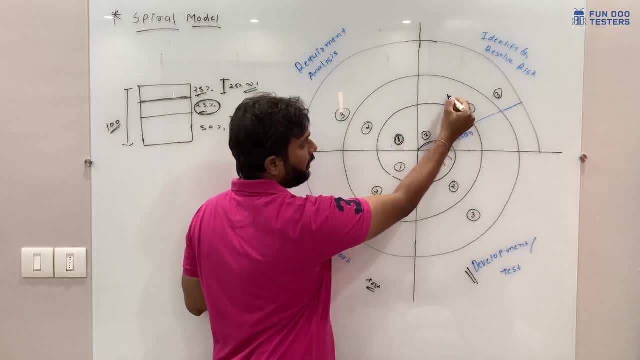 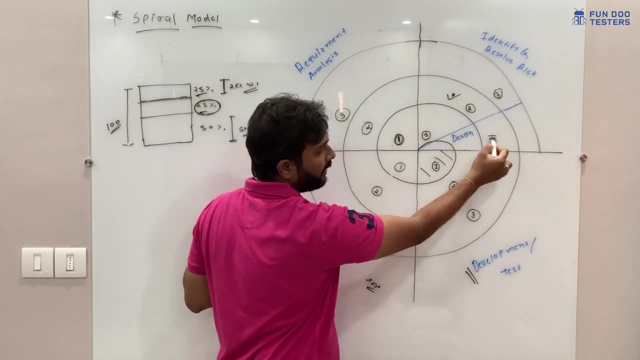 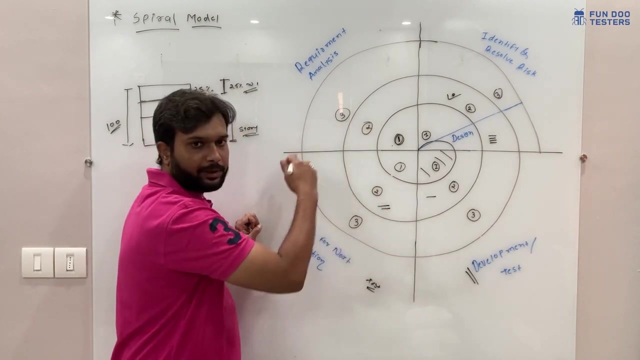 percentage, and then it will identify here: uh, here we. we will be here in the second page, identify and resolve the risk, and we will do the. we will make the design of this page and again, development, encoding and display. so this is how we are moving spirally: one first phase is done, then we are into 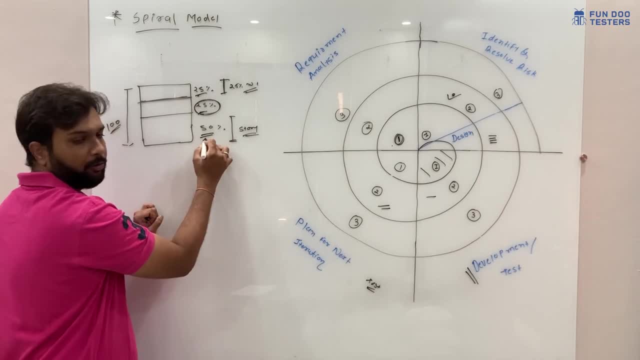 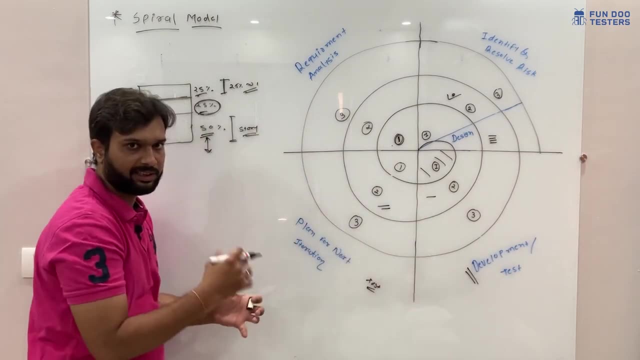 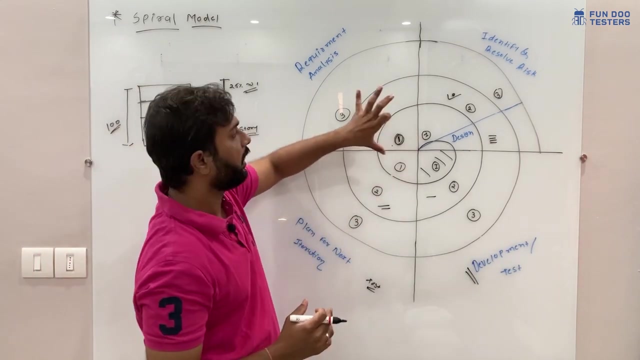 the second phase. one second phase is done. then again we follow the same procedure of this 50 percentage part requirement analysis, risk development and again plan for the next iteration if we have another plan. so this is how spiral model will work: 25 percentage, then 25, then 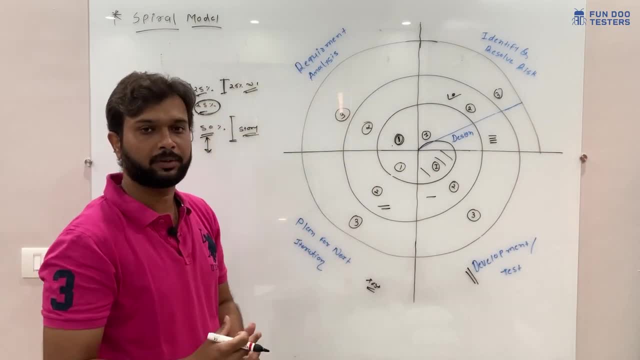 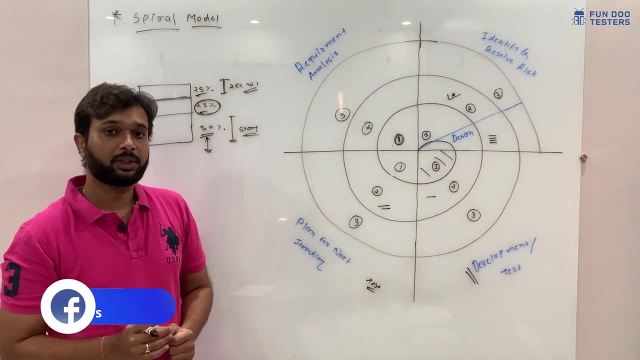 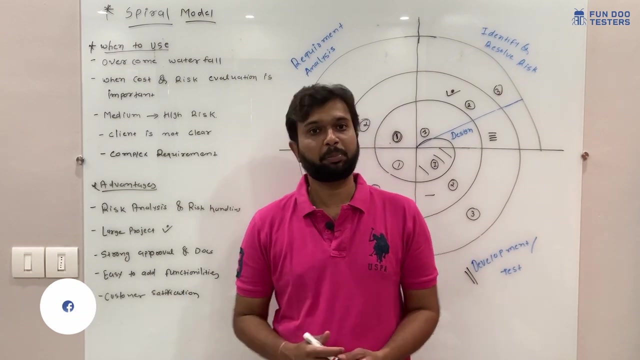 50, or then 10, 10, 10. this is how it works. so i hope, up to this, it is clear. so now we are going to discuss when we need to use the spiral model or what are the disadvantages and advantages of the spiral model. so now we are going to discuss when we should use spiral model. so the first point is: 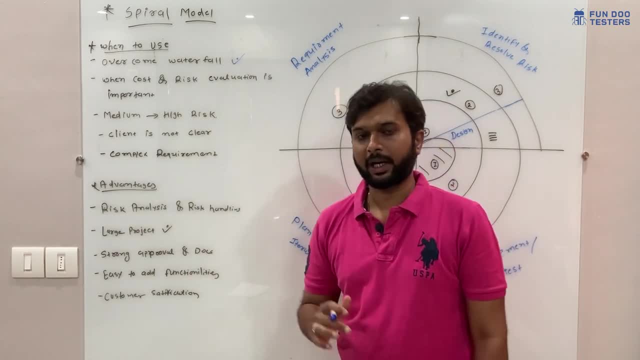 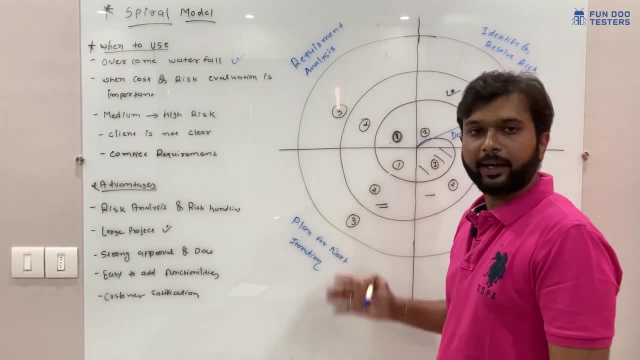 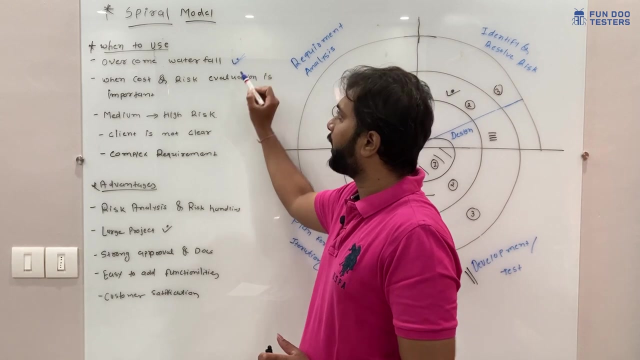 to overcome the problem of the waterfall model. so, as i told, if client is not clear at initial phase, so and later on he can or they can add the functionality. so this is the main purpose: overcome the problem of the waterfall. so in this case we can adopt the. 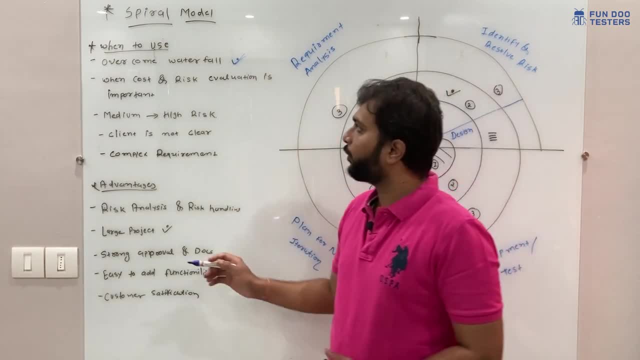 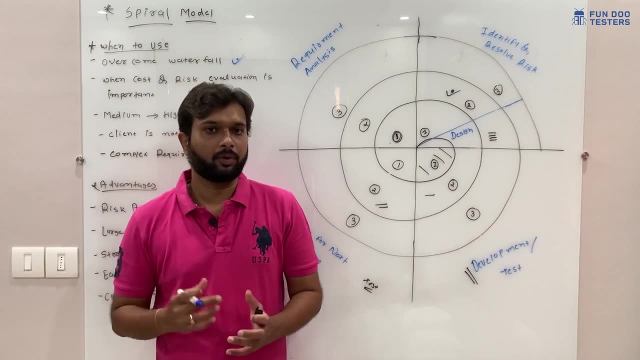 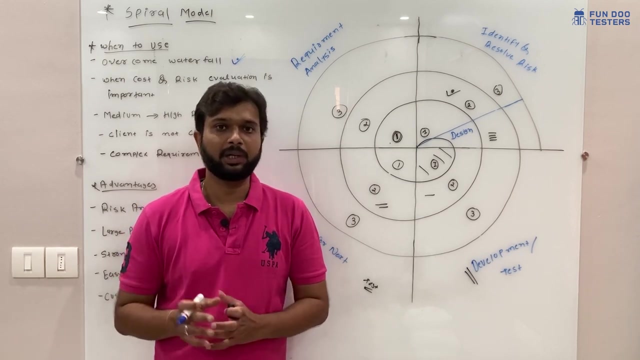 spiral model model or we can go with the spiral model. now, the second point is when cost and risk evolution is important. so what happened? when we are going for? we are going for the large or complex product by that time we need to consider the cost and risk if the product is bigger by the time we 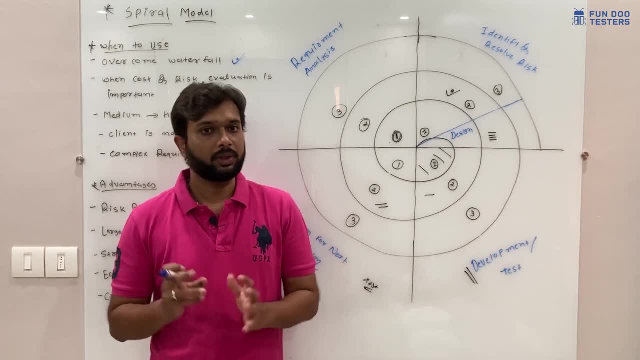 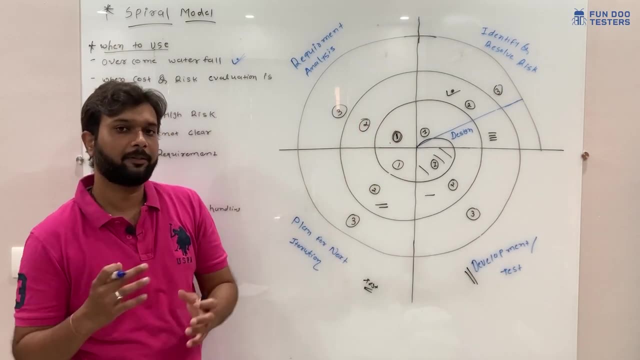 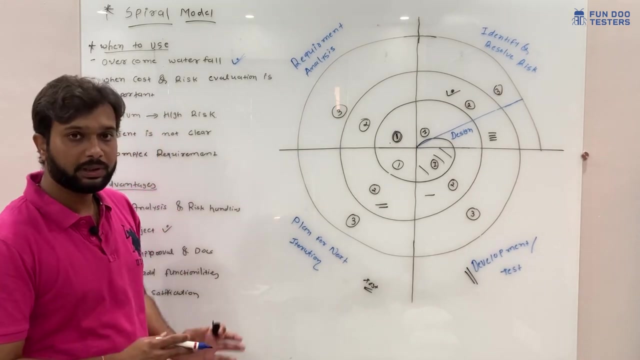 need to definitely come up with the proper estimation or cost. so in that case, if we consider only first phase and later on again, we can identify the cost risk and in this phase we can go with the spiral model. another is medium to high risk product, so this is again. 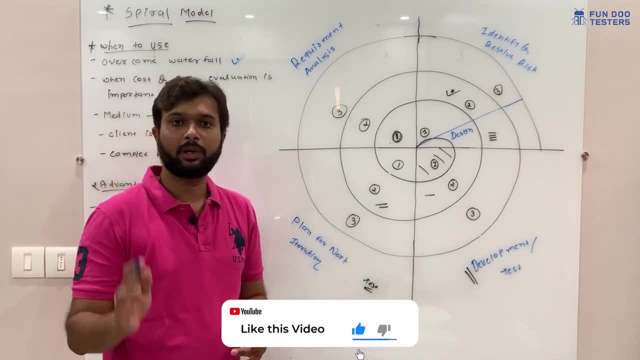 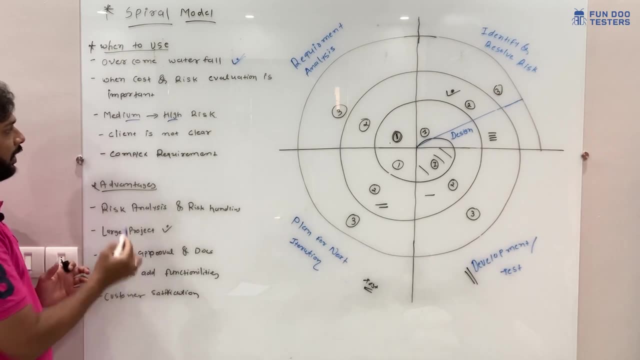 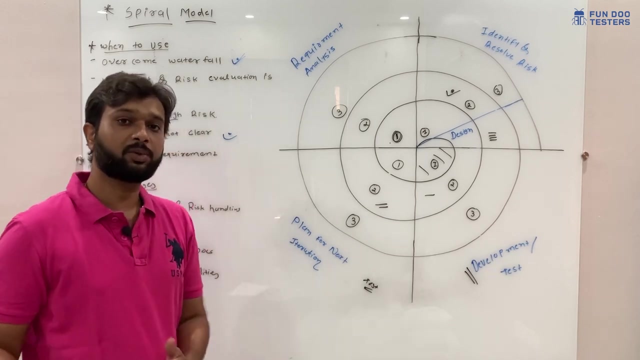 the problem of the overcome of the waterfall model in waterfall only preferable for the small product, but here we can go with the medium or high risk product. now the client is not clear about the requirement. so what happened when, if client is not clear or market is going to change? 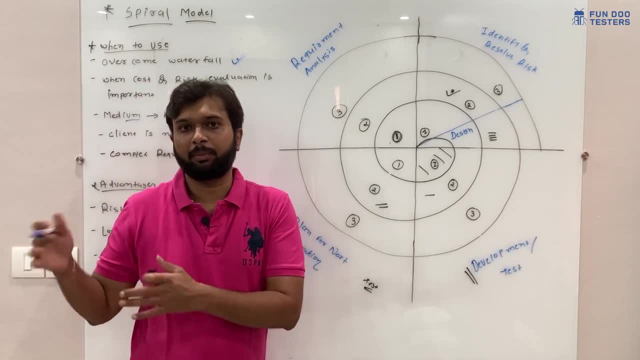 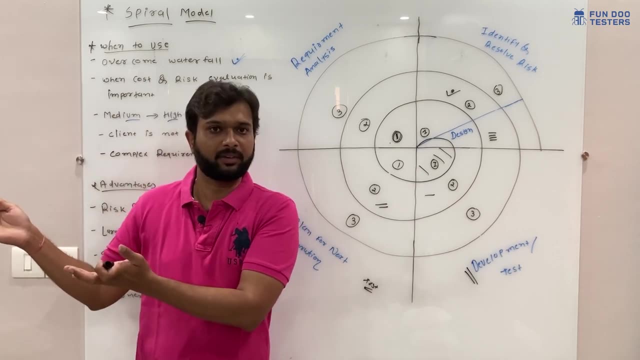 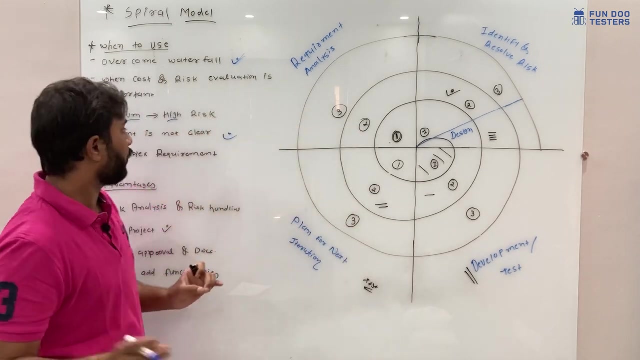 consistently so. for example, in next one year market is going to change. so till one year we can develop some functionality. later on we can move ahead with another functionality or client can add a few more functionality in phase two or phase three. so this is the plus point of the spiral model: when client is not clear or they wants to add. 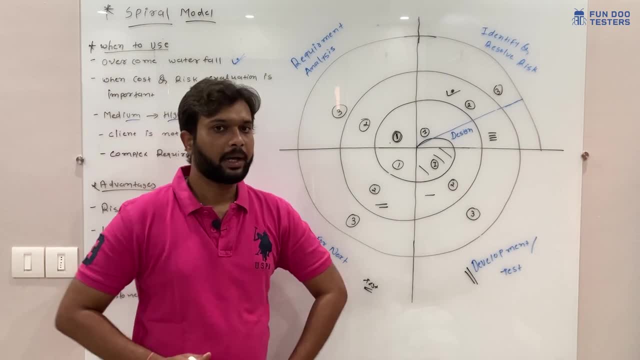 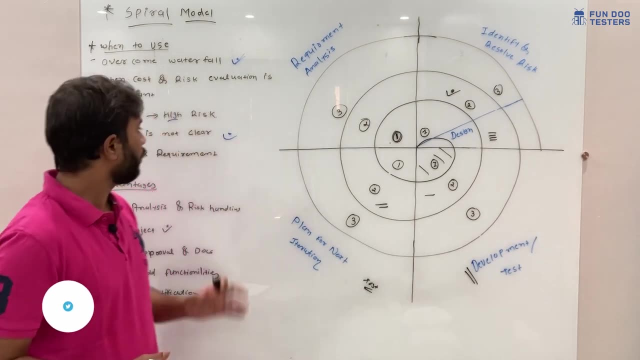 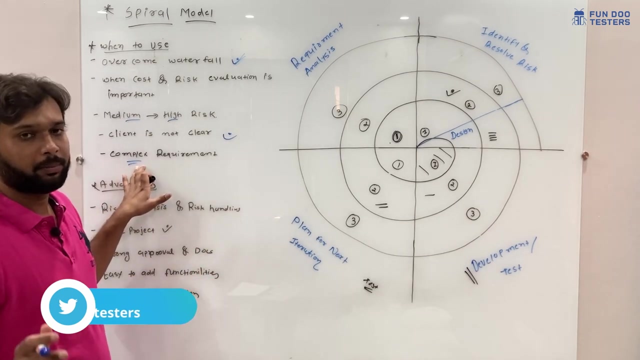 the functionality on later phase. by that time they can go with the spiral model. now, another point is complex requirement. so definitely if product is going to a medium to high risk or large scale product, in that case complex requirement should be by default complex. so in that case we can go with the spiral model. now we will sorry. what are the advantages of the spiral? 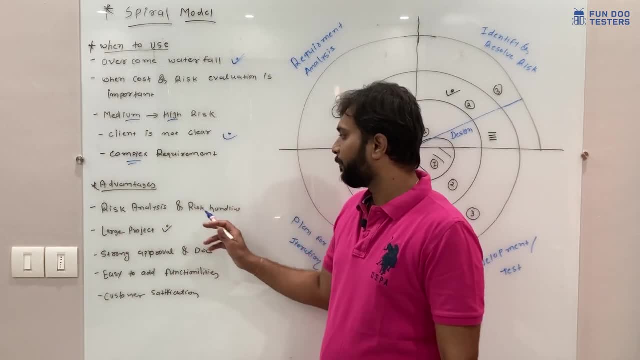 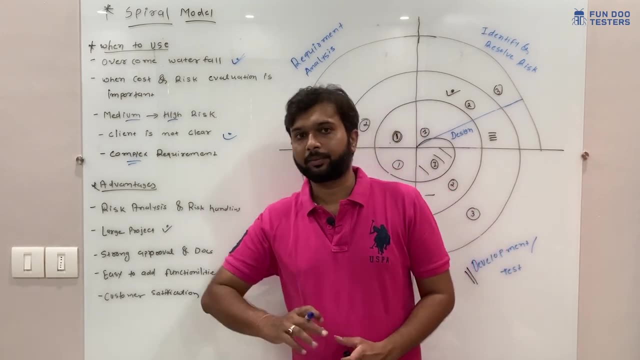 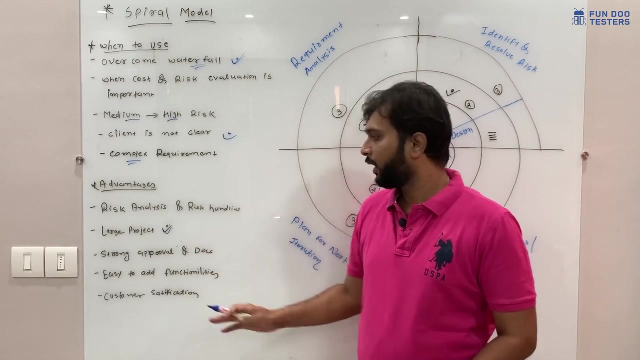 model. so first advantages is risk and risk analysis and risk handling, so we can easily manage the risk. another is large product. so this is again this is the main overcome of the waterfall model. so we can here, we can go with the large product and another is strong. 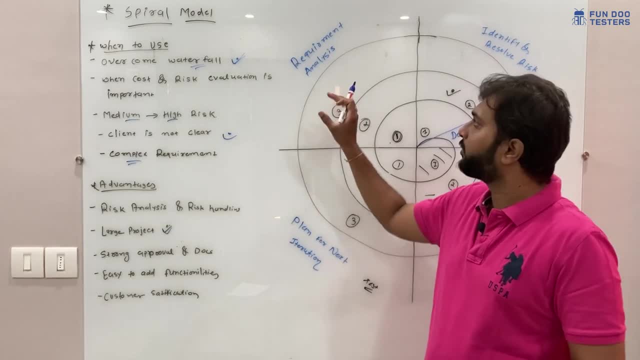 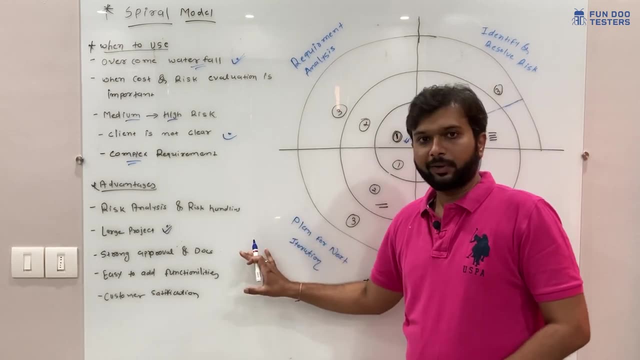 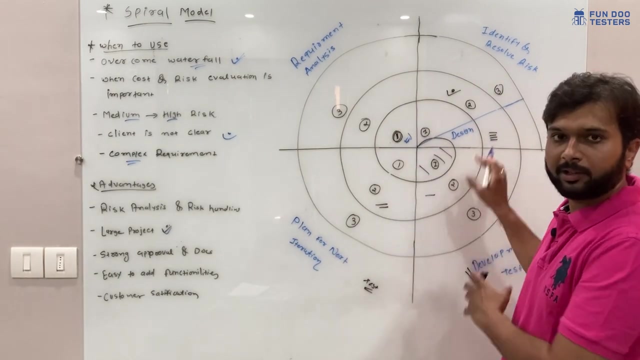 documentation. so what happened? so for first phase, we have completed the requirement here. we completed this phase. so by that time we will have approval as well as the documentation. so here, each and every phase, for small, small chunks, we have documentation. so every phase we need to go with the documentation phase and legal term. so end of the project or end of the one or two. 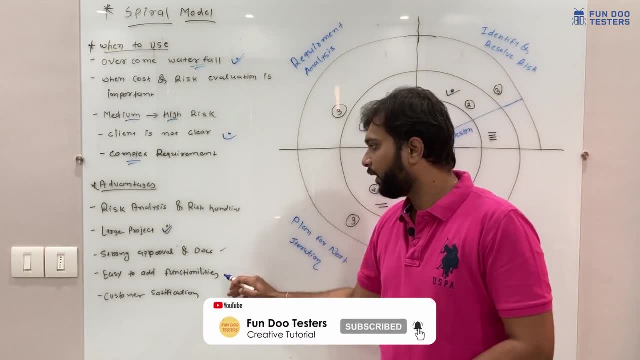 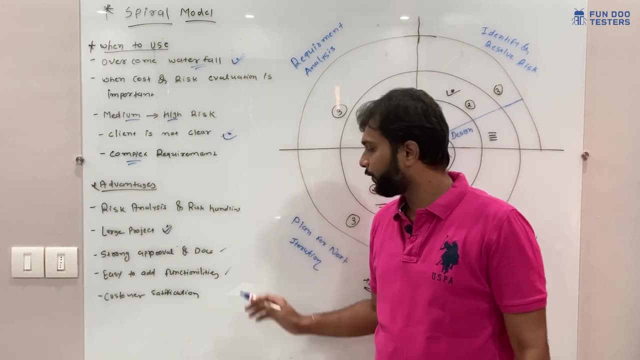 phase. we will have a strong documentation later on, easy to add the functionality. so that's what we have discussed here. client is not clear, so in that case we can easily add the functionality in waterfall model. what we need, what we have to do, we have to rework, we have to go from. 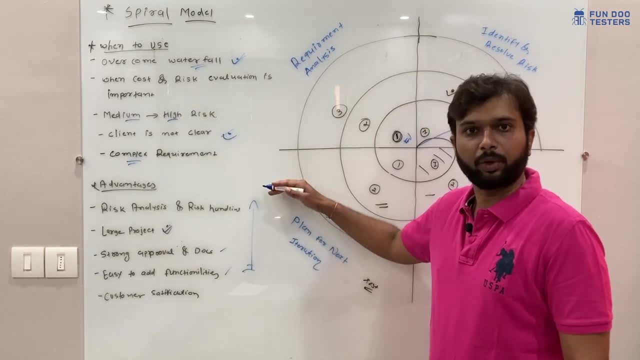 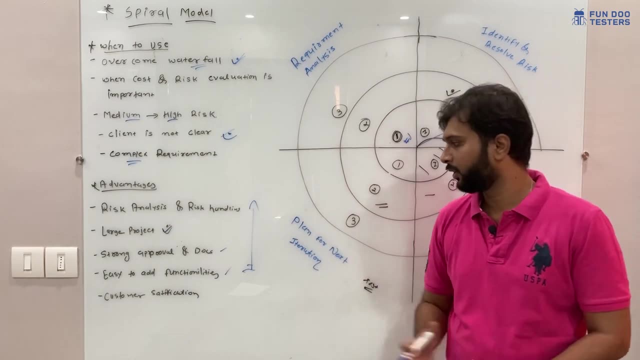 the lower stage to the upper. we have to go to the backward direction. but here what happened? we can next phase, we can take the new functionality, so no need to worry about the backtracing and customer satisfaction. so by definitely customer will satisfied with this model. what happened if? 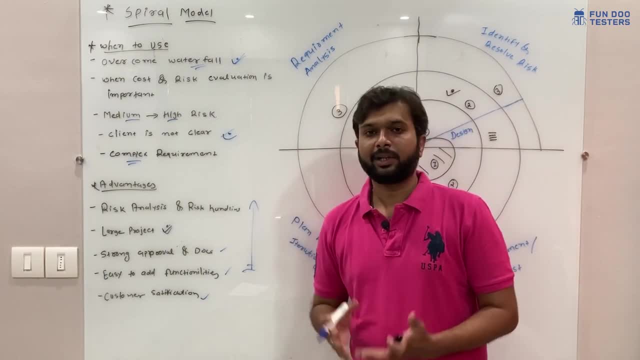 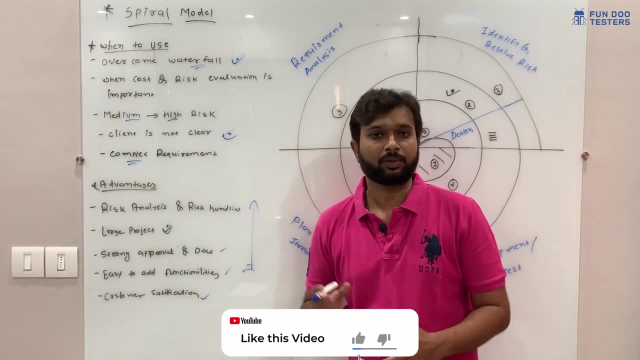 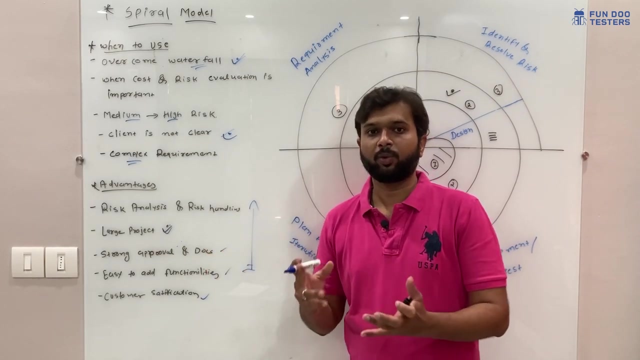 customer want to add the new functionality in simple term, only if we are going to purchase, or if we are going to purchase new t-shirt or jeans. we are not satisfied with that product. so what we will do, we will return that product. so this is the software, big chunk of application. so definitely after two months or three months we 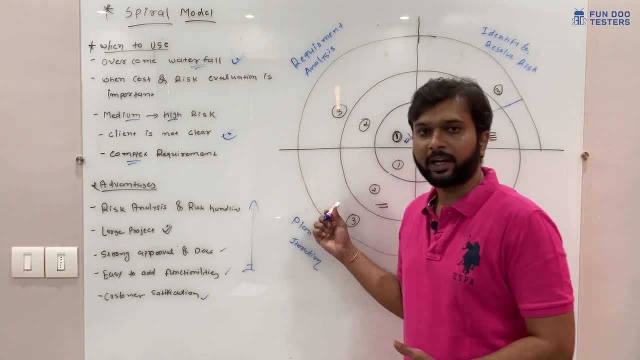 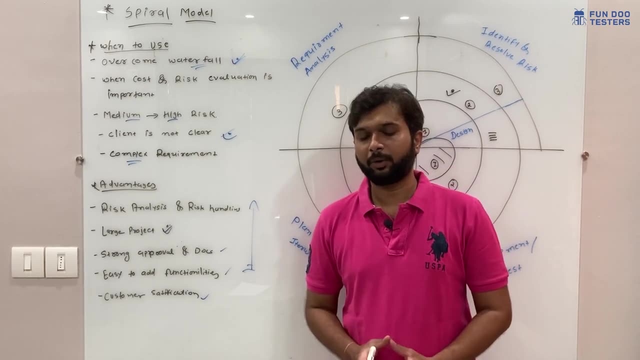 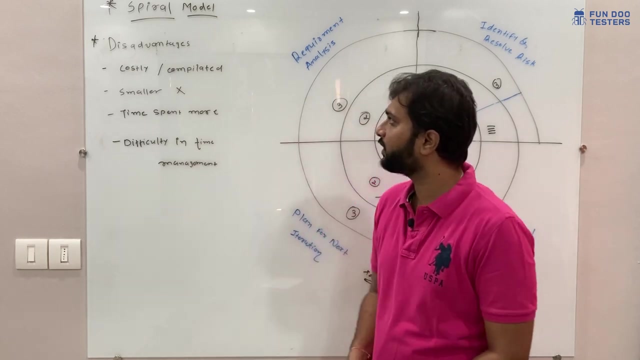 will or they will come up with the new suggestion and easily we can adapt here so customer will satisfied with the product process and model. so this is the main of M of the spiral model. so now we will discuss about the disadvantages of the spiral model. so first disadvantages: is costly and